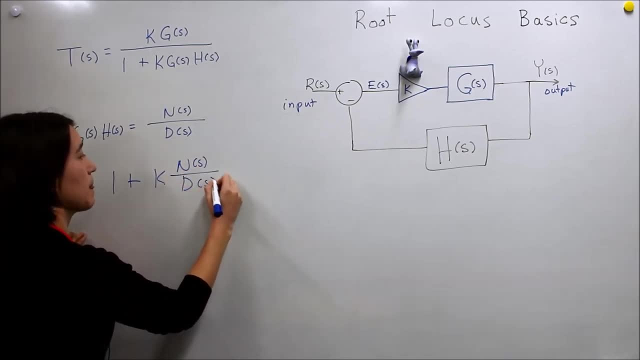 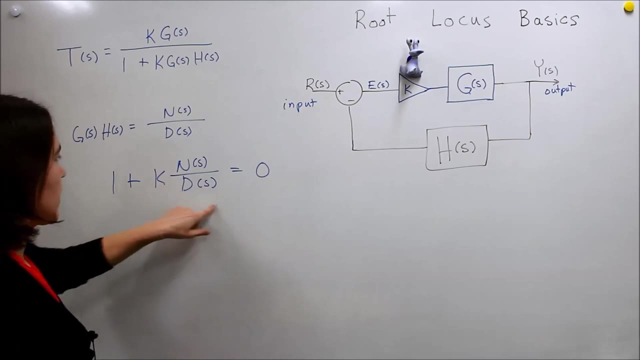 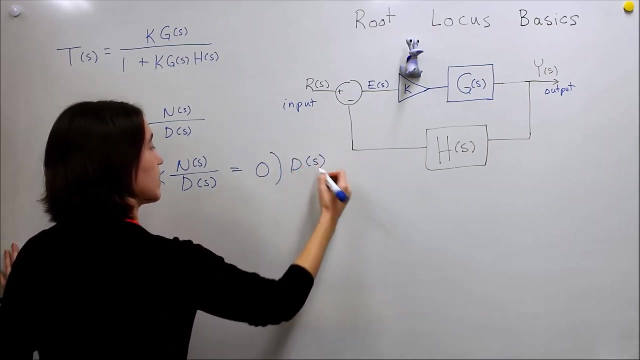 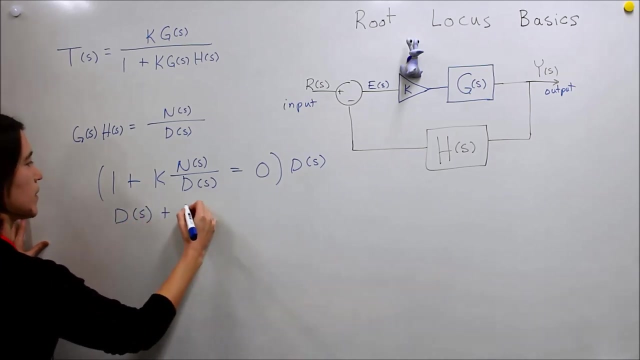 some expression in terms of S and some denominator expression, And this has to be equal to 0 to evaluate the poles. Now we usually want to get rid of any S's in the denominator, so we can multiply this whole expression by D of S and then we can solve it here. So 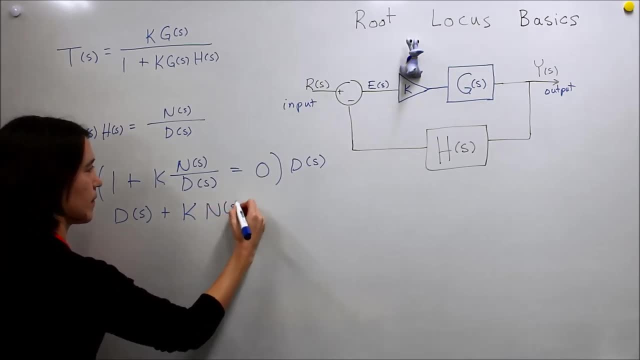 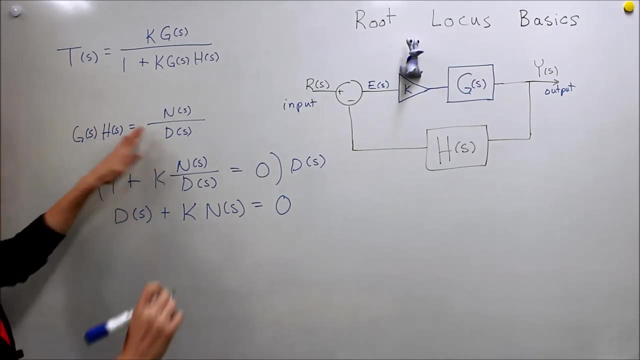 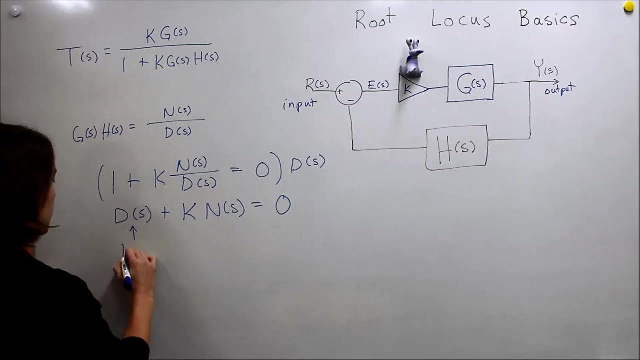 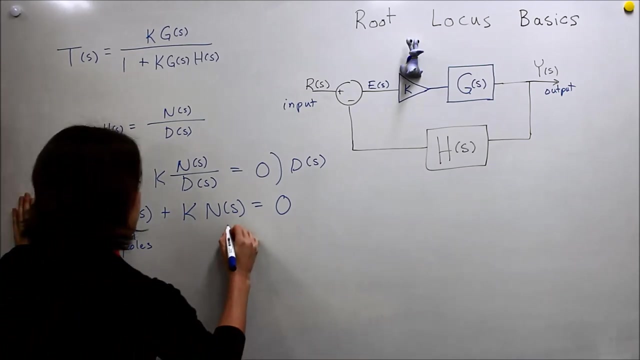 here we have our K times N. S equals 0. So we can get it in this form And remember our denominator here. these would be the poles of the systems, So these would represent the poles and the numerator represents the zeros of this system here. And what we're going to do is we're going to vary K, starting from. 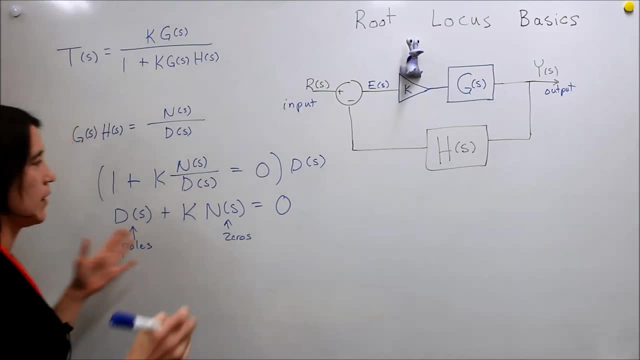 0 into infinity. Look at this equation though. Think for a second. What if K is equal to 0?? So if K is equal to 0, our expression simply becomes D of S is equal to 0.. So the poles of this? 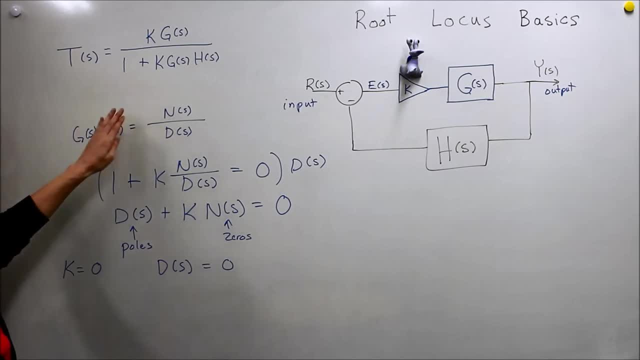 system of our G times H. the poles of that system are the poles of our closed-loop system. OK, Then let's take the other extreme. So if K goes to infinity, so if the K goes to infinity here, these are essentially going to completely be ignored, And then K dominates and all. 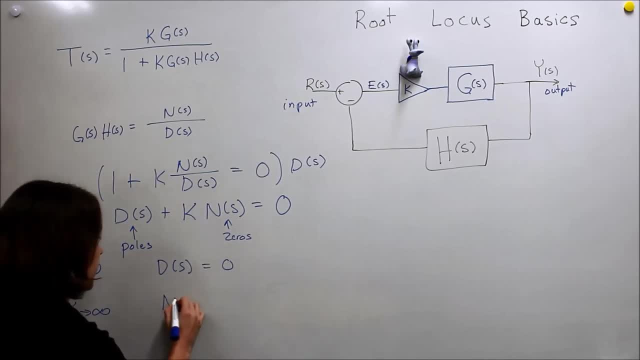 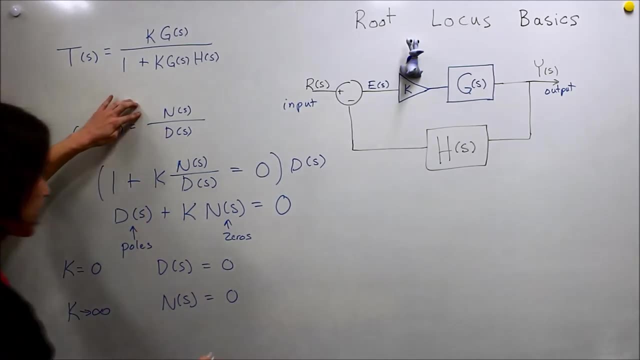 we have is N of S is going to be equal to 0. And these, this is the numerator. so these are the poles, sorry, the zeros. These are the zeros And these are the poles. the other example we gave. this is the poles of our G h here. 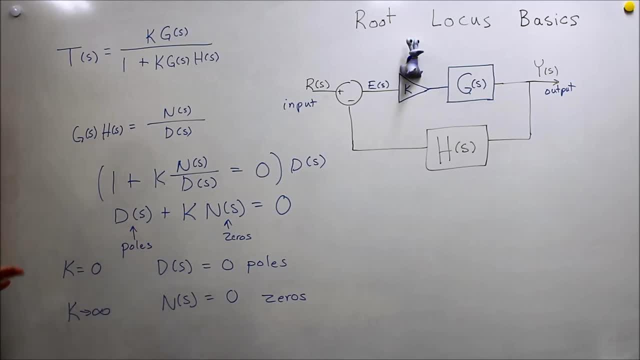 and these are the zeros. So, in a sense, if K is 0, the poles of this thing are our closed-loop poles, OK, And if K is infinitely high, the zeros of this system become our closed-loop poles. So we're going. 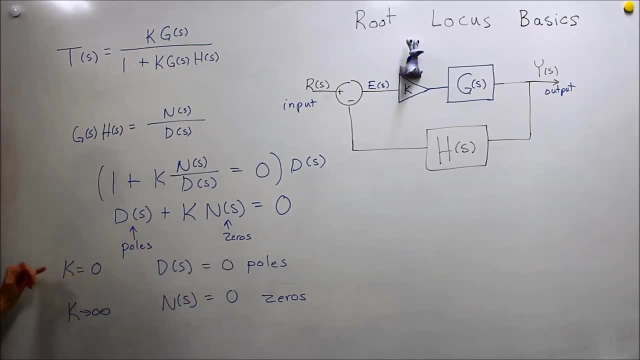 to use those as one our starting points. So, when k equals 0, we're going to start from this point, from the poles of our gh, and we're going to end because we're going to take k from 0 all the way to infinity. and 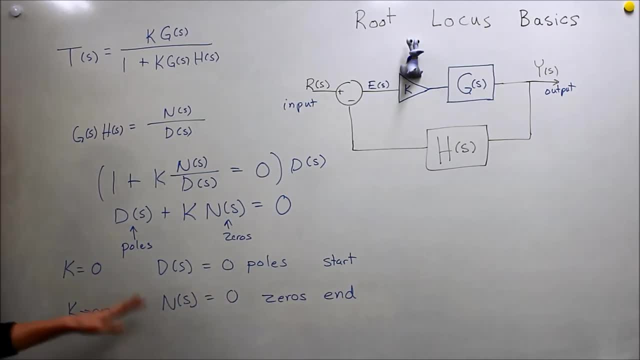 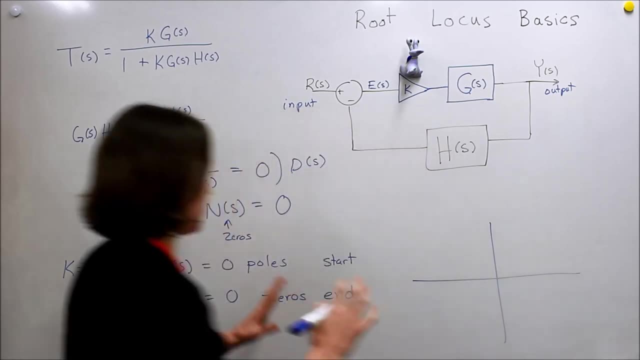 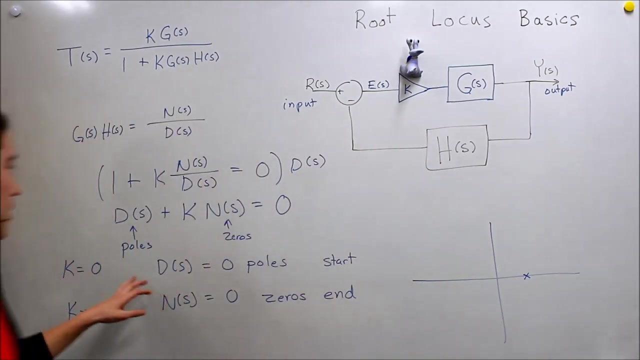 we're going to end at the 0s of the system. okay, So we're going to draw that on our S map So say we have. I'm just going to make an arbitrary example here. so if we started and we had an x, a pole, a pole from our original system here, and we had a 0 here, this would 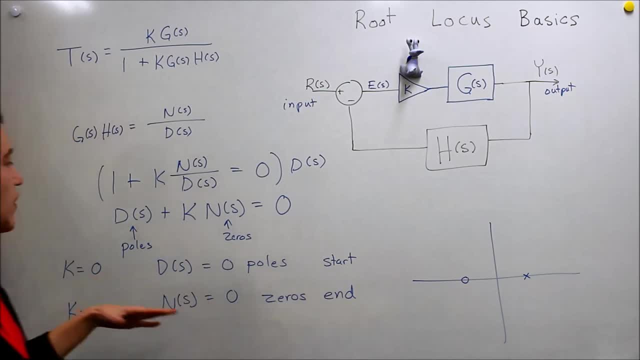 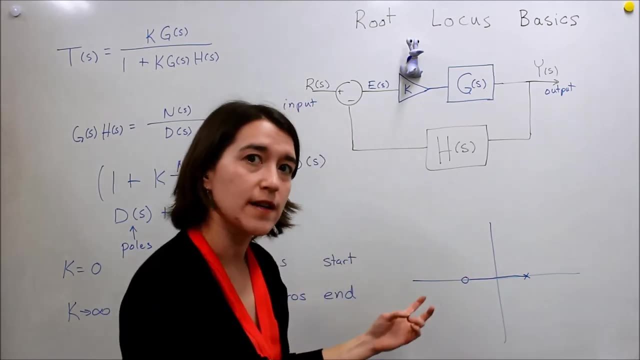 be our starting point and our end point. Also, note that we're going to have a bunch of different lines going through here, so this line will look like this: That's one branch is what we call it. so this is a branch, Okay. 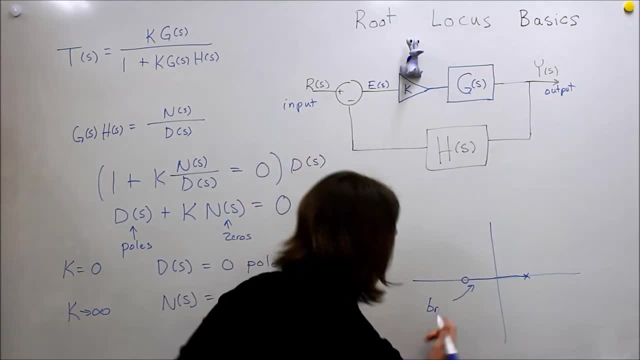 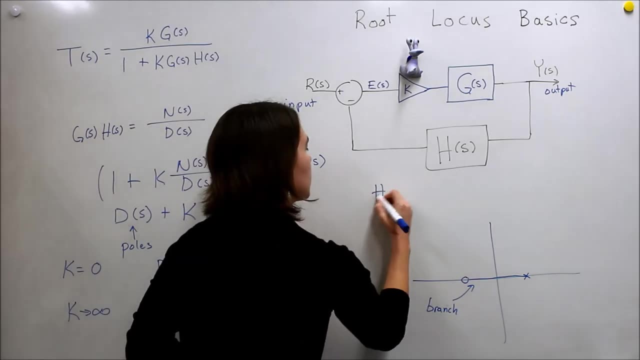 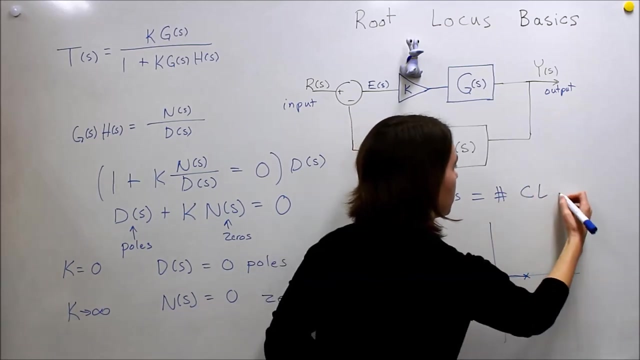 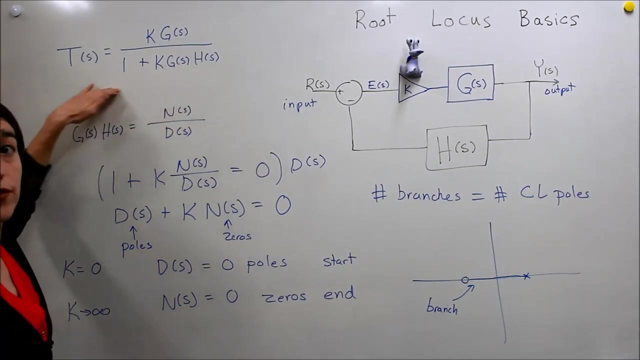 Oops, branch. and the number of branches for a system is equal to the number of closed looped poles. So if we have, it's the closed loop right. so it's this full expression. So if we have 1, we'll have 1 branch. 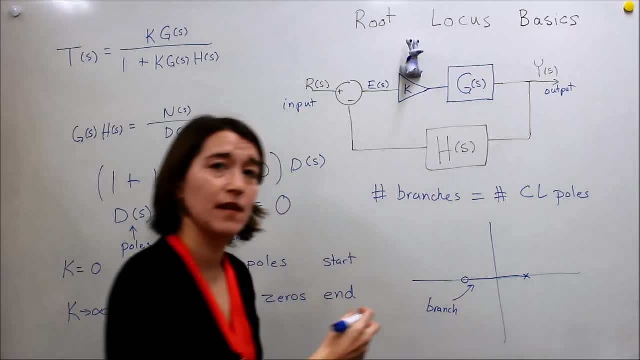 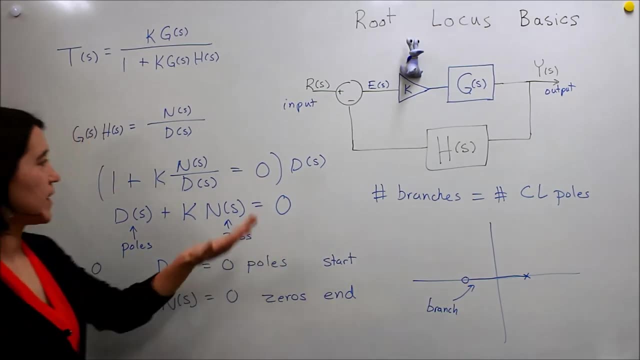 If we have 20, we'd have 20 different branches. Okay, So we have 20 different lines that are going to map from k value equaling 0 to infinity. Okay, so this is the basics. The important things that you need to remember here are the number of branches that we're. 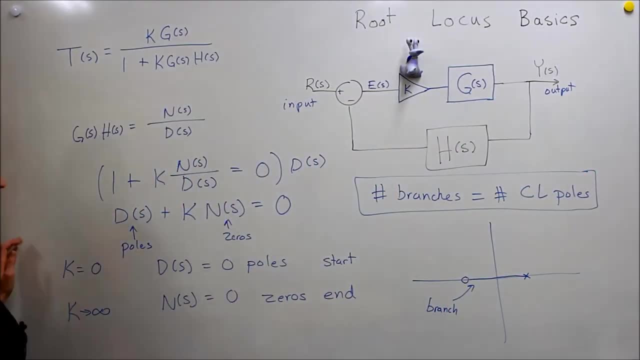 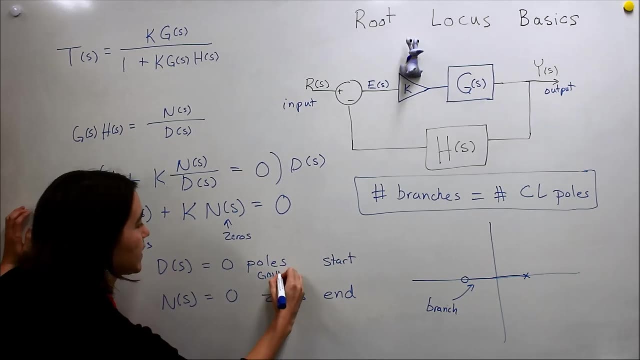 going to see are the number of closed looped poles, and we start at the poles, so poles of, and I'll just write it here again- G, S, H, S, that's where we start and we end at the 0s of our Gs. 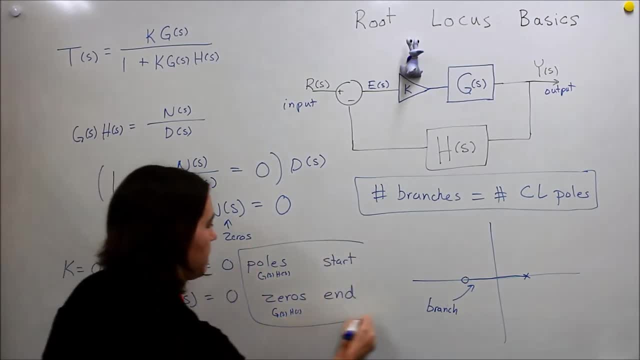 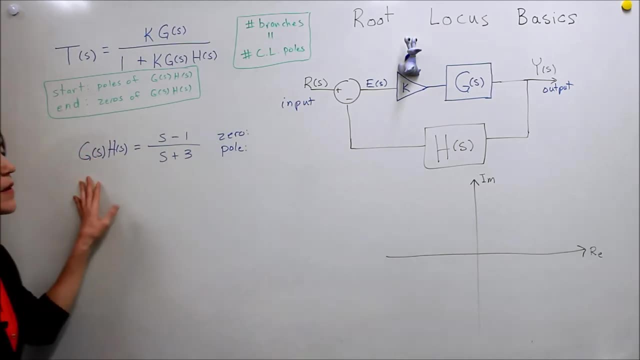 H, S, H S equation. alright, Now let's take an example. So let's do a very simple example of this is the equation for G and times H, here, just S minus 1 divided by S plus 3.. 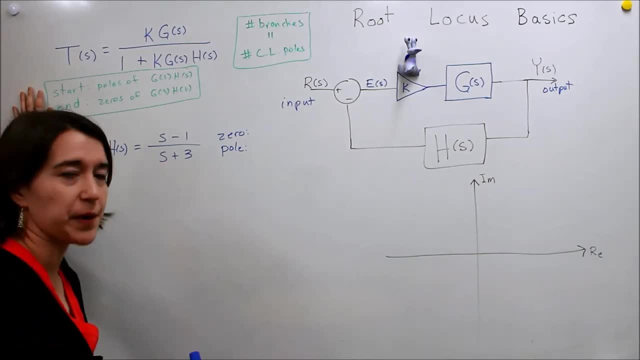 So first thing we need to do, remember, we need to find our starting point and our end point. So to do that, we look for the poles and 0s of our G times H, G times, H expression. So here it is: our 0, we can see easily, is 1, positive 1, and our pole is at negative. 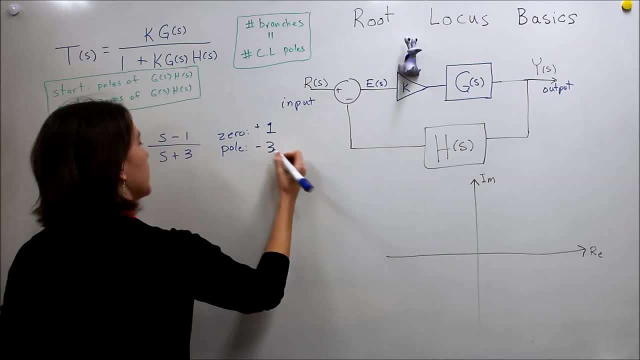 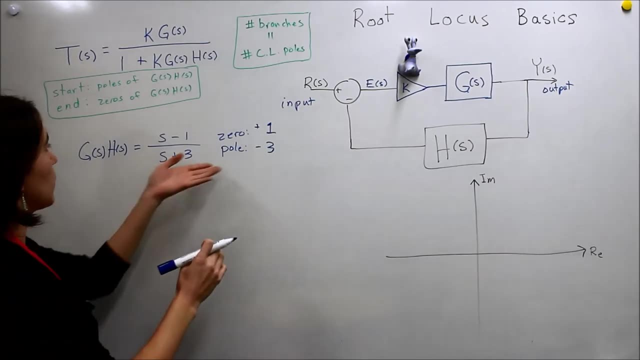 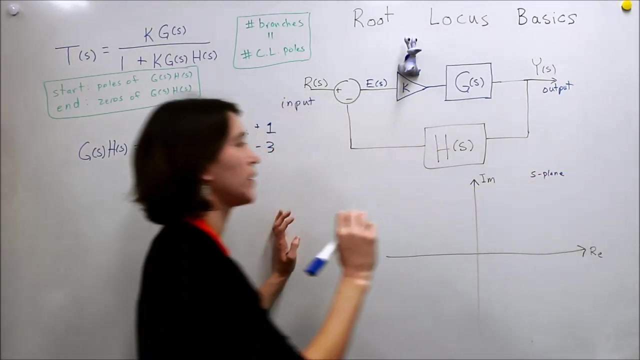 3. Okay, And note, this would be a stable function on its own, so that's good to know, And so what we'll do first is: here's our S plane, and we will simply draw those two points on the plane. 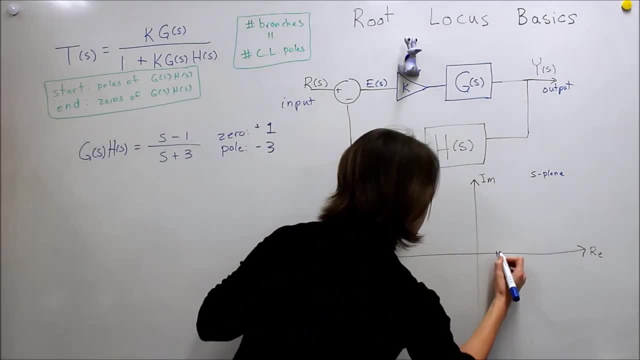 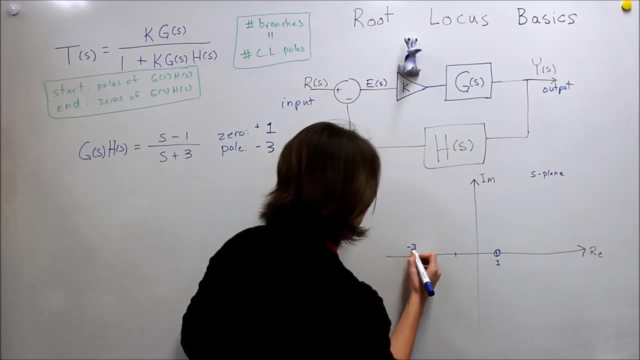 Okay, So 0 at 1, and cos 1 of our 0 here and then at negative 3,. so 1,, 2,, 3, so put it up here. negative 3, we put our pole. 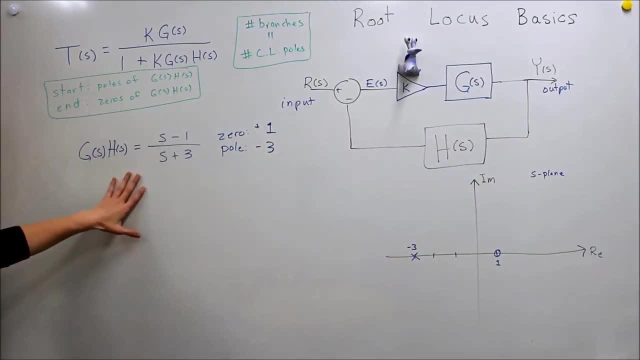 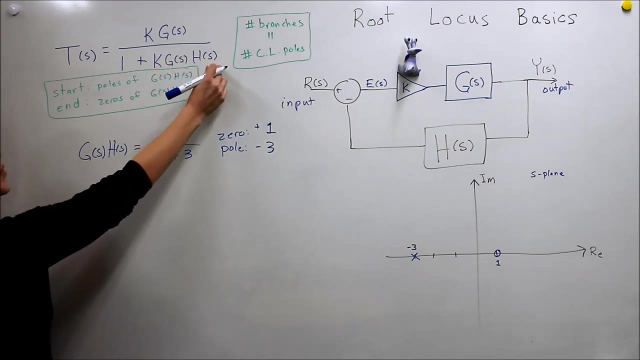 And let's check the number of branches. Well, in this system, we're going to have just one pole, And if you're not quite convinced of that, let's actually multiply it out. So if we did this multiplication out- and I'm going to skip one step- 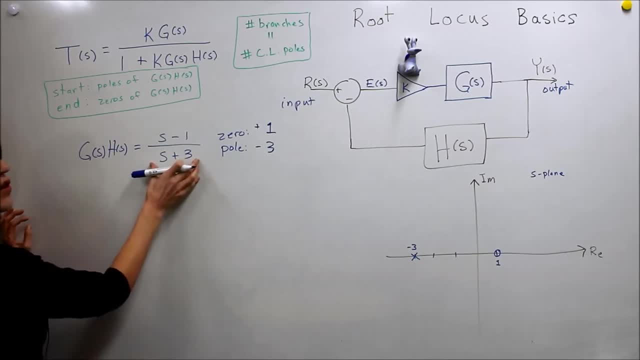 But so we're going to have one pole. Okay, So we would. we know that this denominator would be multiplied and end up over here. So we're going to do that: S plus 3, right, the pole, the denominator of this expression, plus k times the numerator. 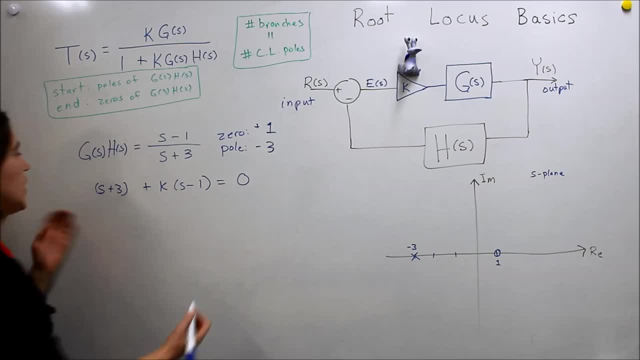 S minus 1, is equal to 0.. And so here the highest order is S, here the highest order is S, and so our number of poles in the closed-loop system is simply 1.. Okay, And note, most of the time we are dealing with properties. 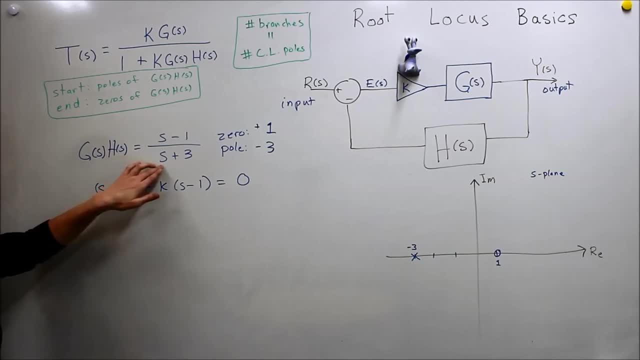 We're dealing with proper functions, So usually it will be the same magnitude as the denominator here, but if you're not sure, you can always go through this and check. Okay, So here we have just one pole, so we will have number of branches, one closed-loop. 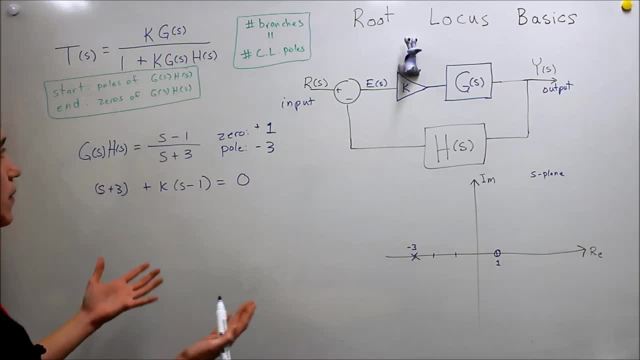 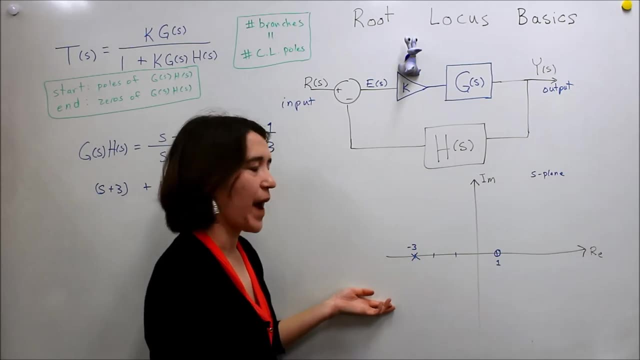 pole, so we'll have one branch. Okay, So we've followed these rules. looks great. We've drawn this on our S-plane. Now the next question is: what path does this take? We know we start here and we end here. 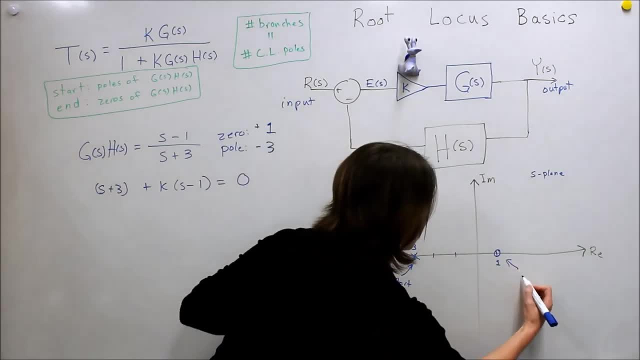 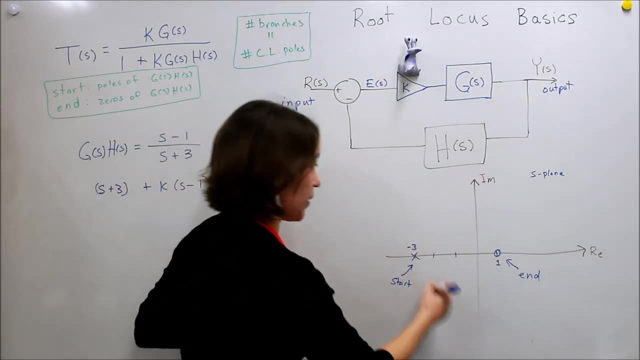 So what path does this take? We know we start here and we end here. Okay, But which path do we go on? Do we go straight across? Do we go up and over? Do we go down? Do we go all around the map and eventually end up there? 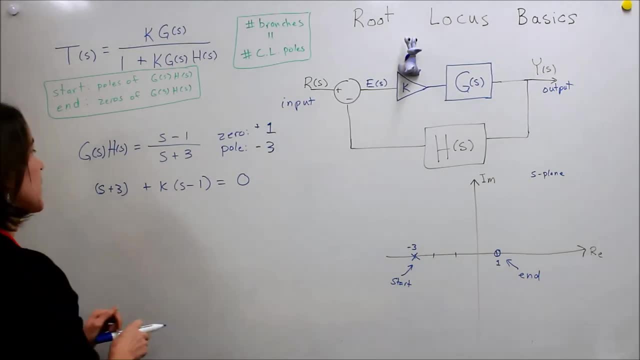 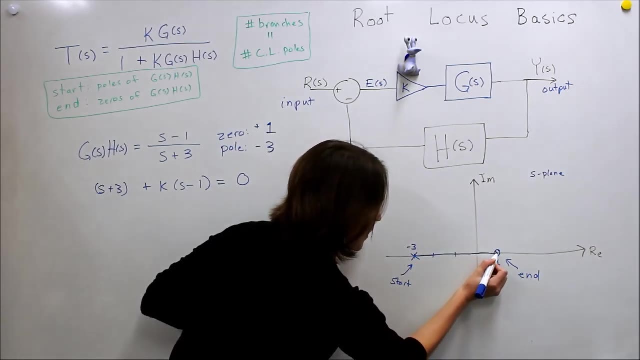 That's a good question. That's the slightly harder one to explain. I'll tell you the answer. What we're going to do is end up just going straight across the real axis here, And so that will actually end up being your root locus path, and usually you draw some. 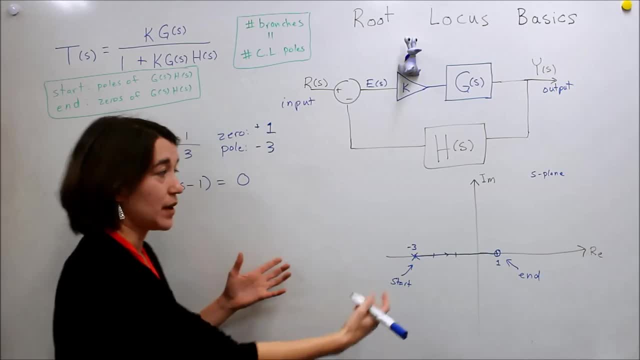 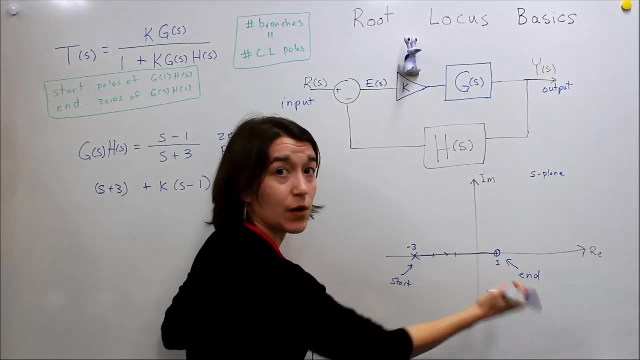 little arrow just to indicate We draw the X for the start, meaning the pole of the system, and the zero. so you know which way it's going, based on the X and the zero position. But I'm going to try to explain this. 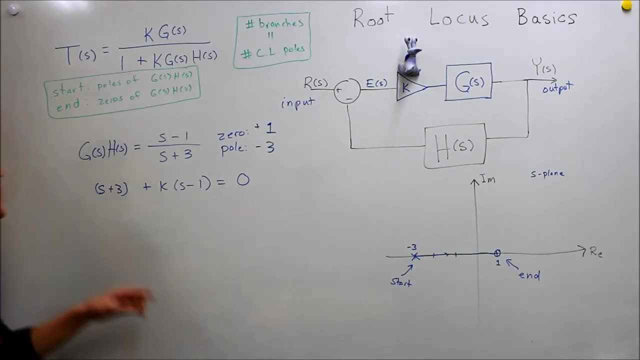 It's a little bit hard, but the other thing that we need to remember is we derived this last time, The angle of this expression, so G of S, H of S, has to be equal to 180 degrees. Okay, Okay. 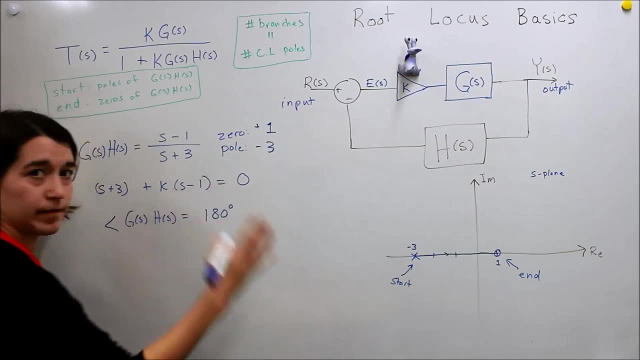 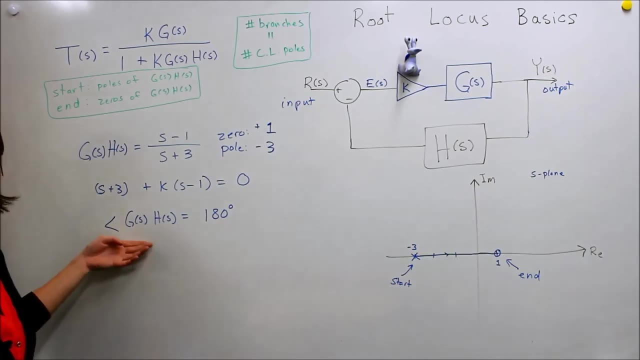 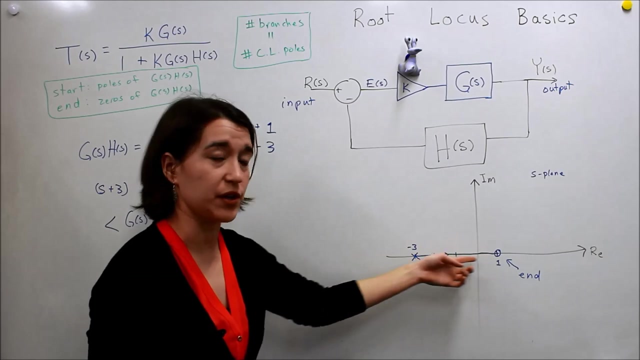 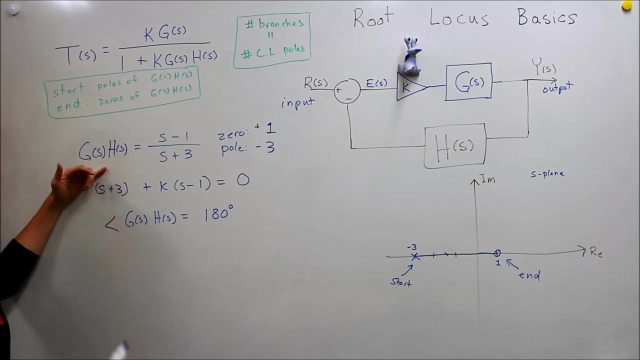 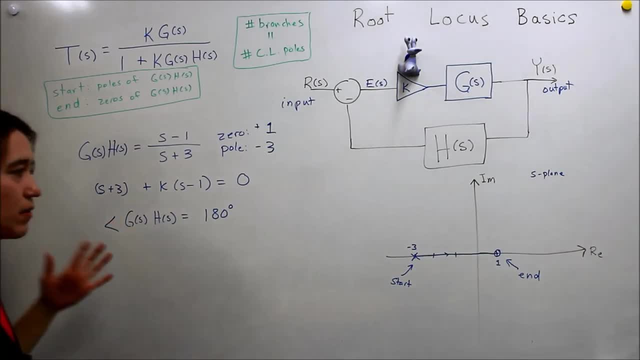 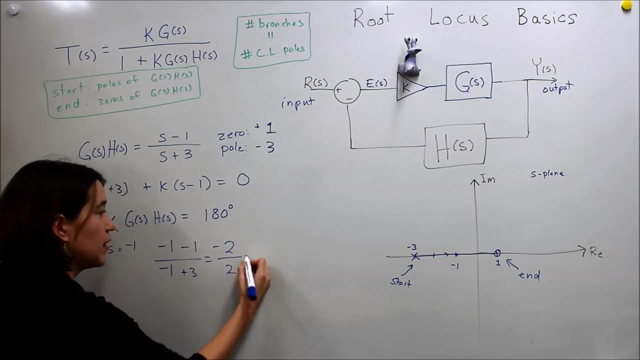 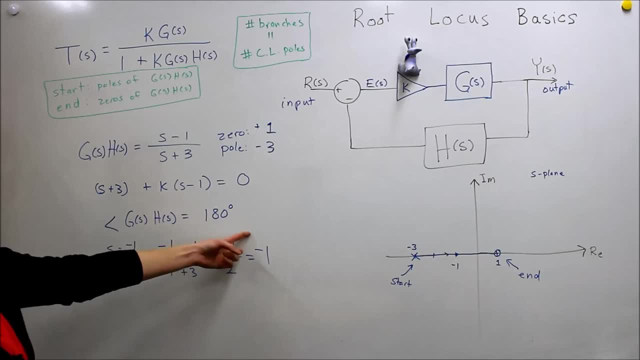 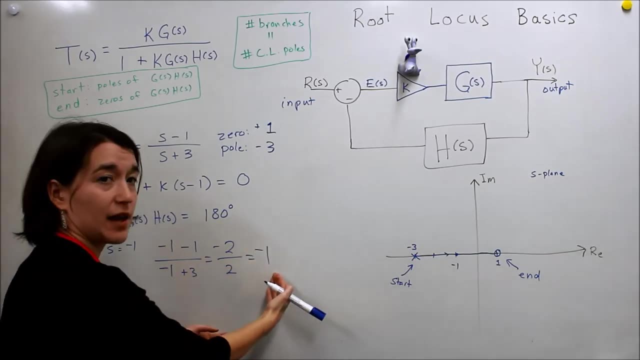 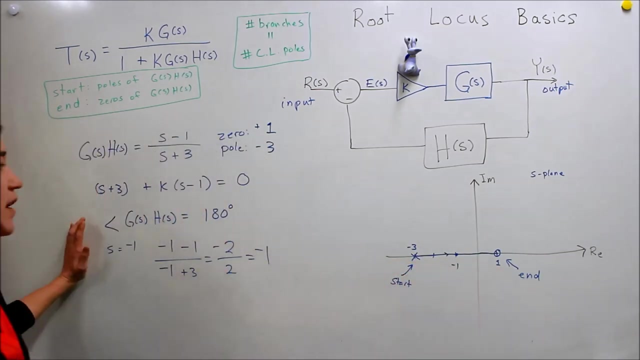 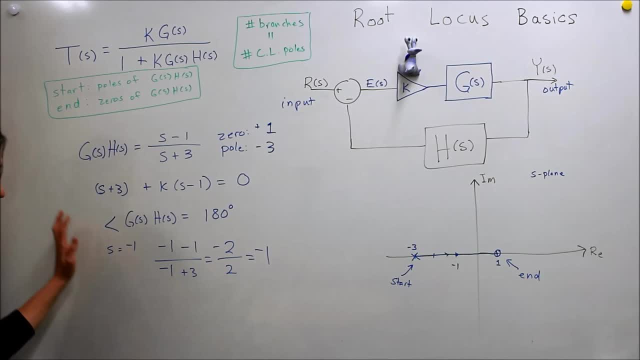 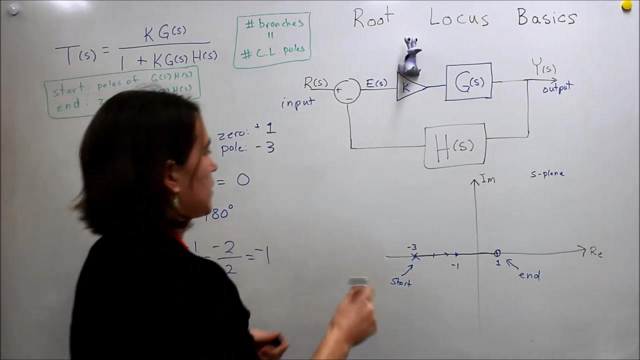 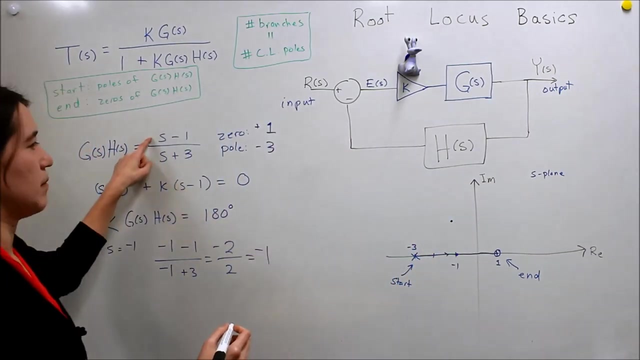 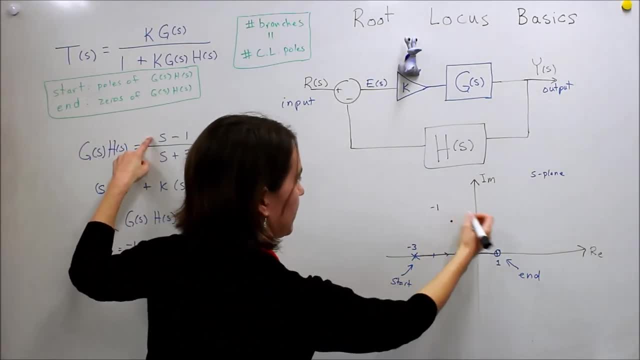 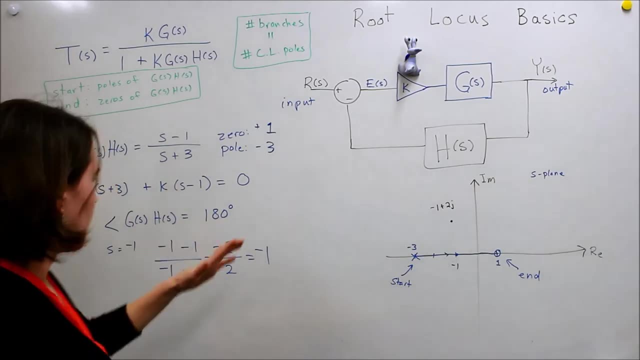 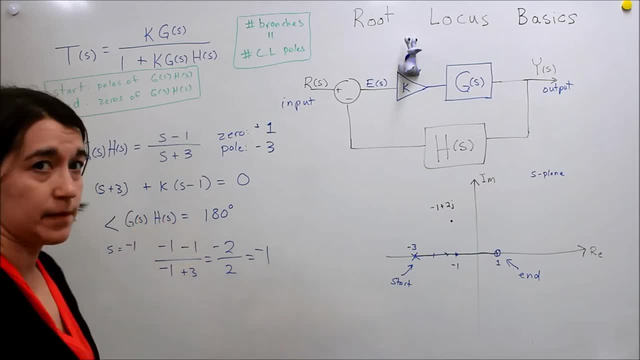 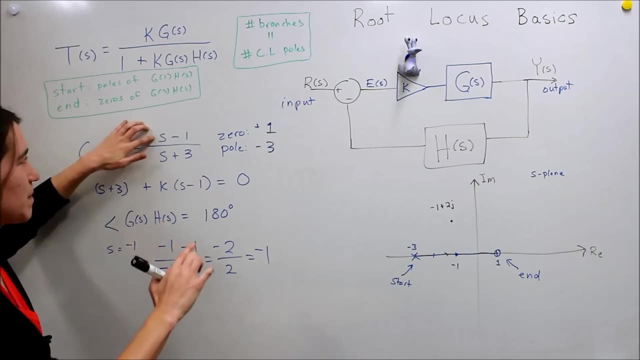 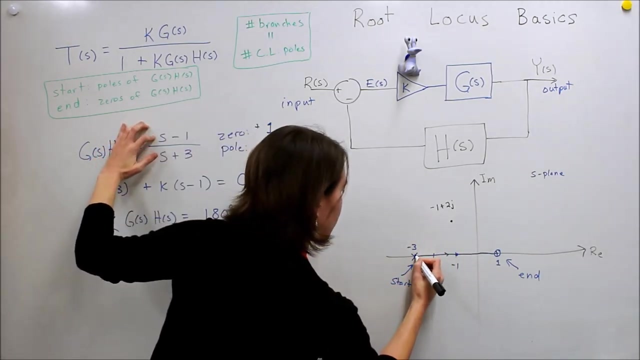 constraint and you can see if it meets this or not. Another way to visualize it is if you kind of go back to your vector math, this s minus 1 is actually the same as if you put this point in here. it's the vector from this point. 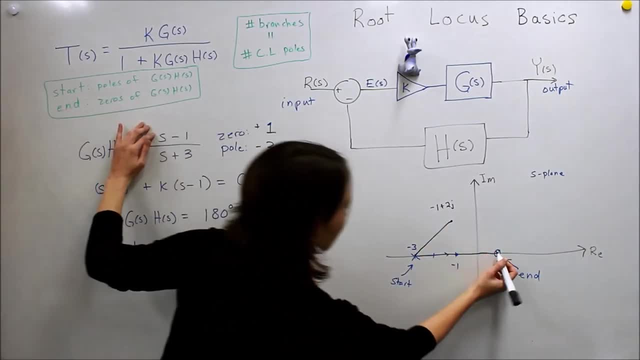 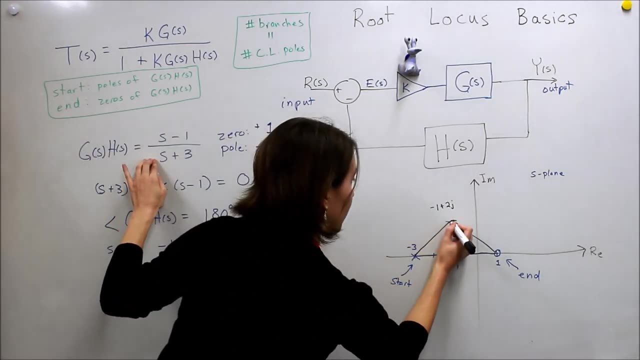 this pole. I'm sorry, that's the s minus 1, it's actually going to be this one, this pole to that point, and since s is the same, we'll also look at this vector. So it's the vector from the pole to the point that you're trying to test. 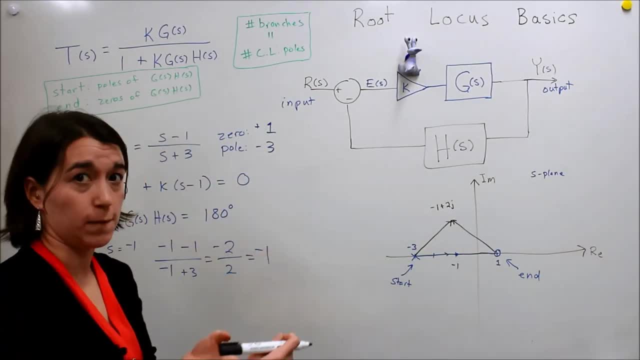 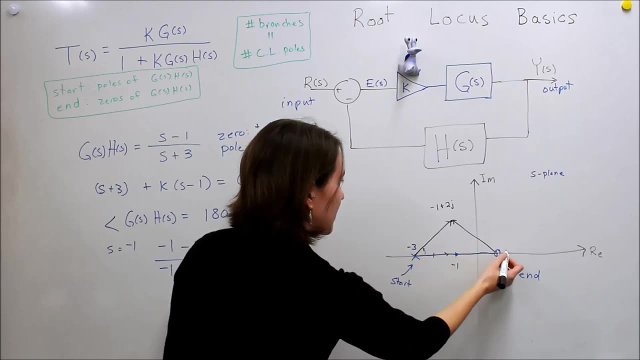 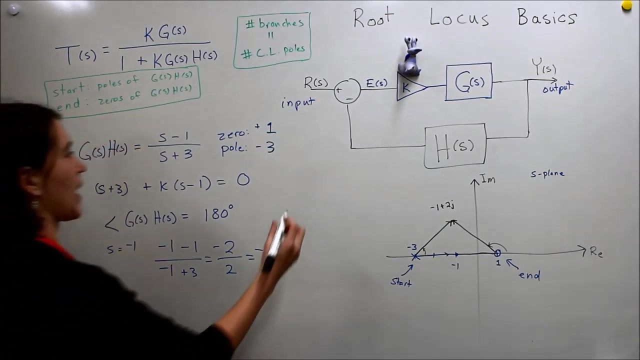 And that vector one has a magnitude and also has a pole- sorry, magnitude and an angle. Okay so this has an angle here, some value, and this also has an angle here, some other value. And when we, if we wanted to divide two values, so say we have, I'm not going to give the 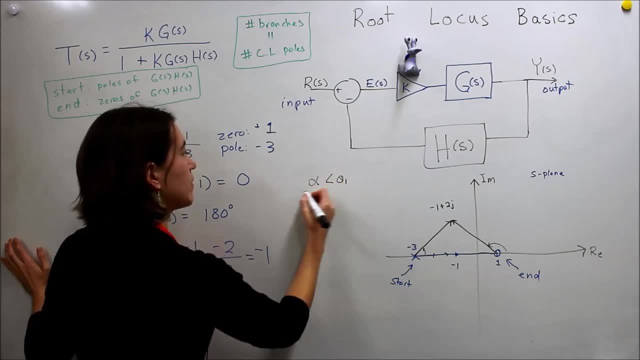 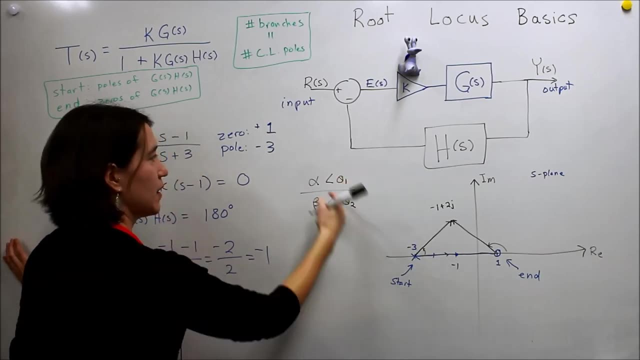 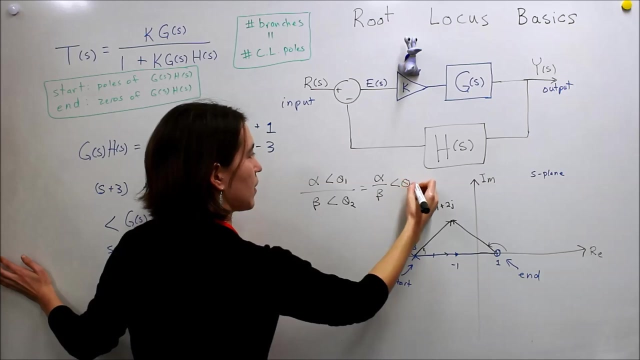 actual value, just alpha and some angle theta 1, and we have a beta and some angle theta 2, if we want to evaluate these, we would get alpha over beta and we actually end up subtracting the angles: the theta 1 minus theta 2.. 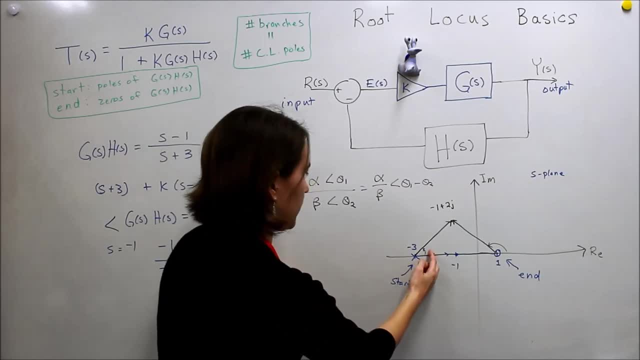 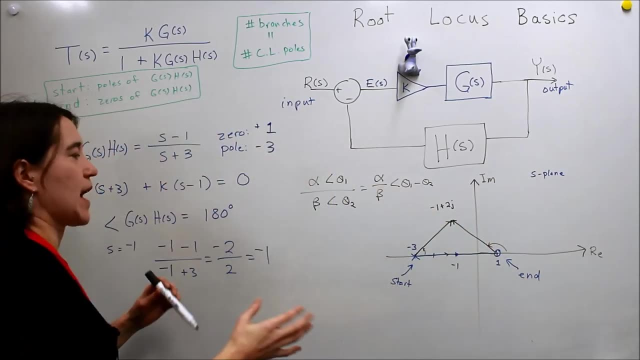 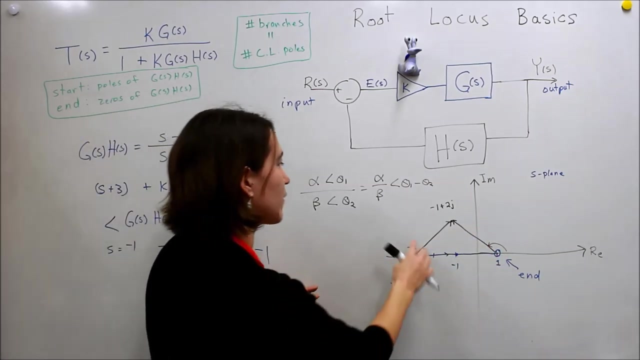 So if we look at this value, So if we have, we have this value and we subtract this value, in order for the angles to work out, it has to be exactly 180.. If you go through the math of this, you'll find that it will not be 180 for any of these.